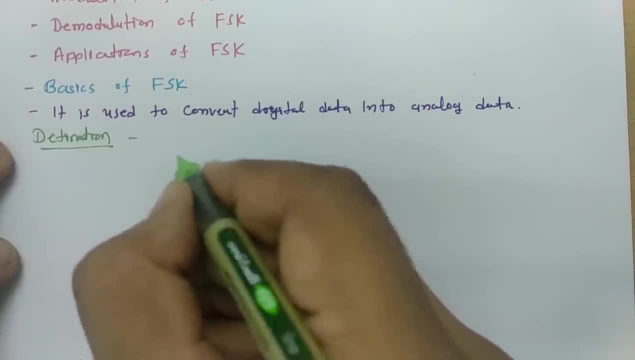 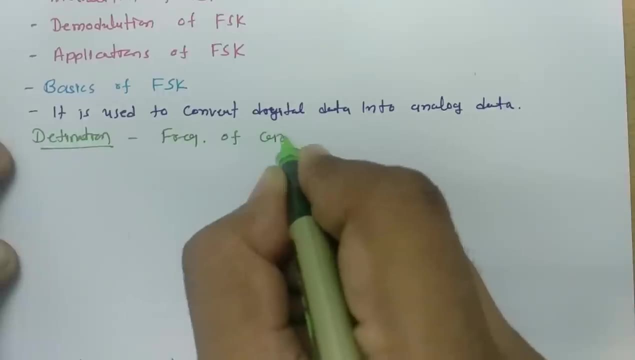 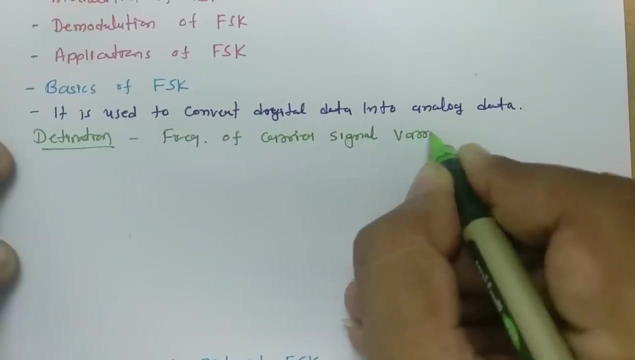 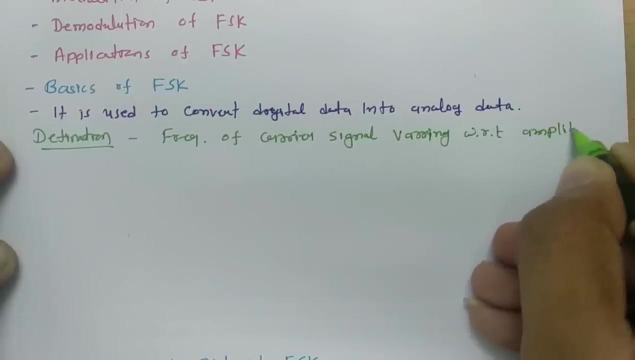 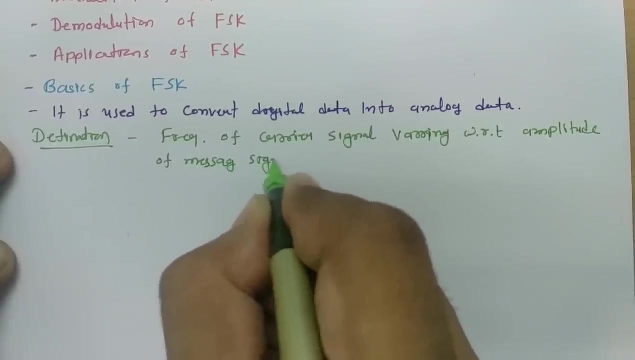 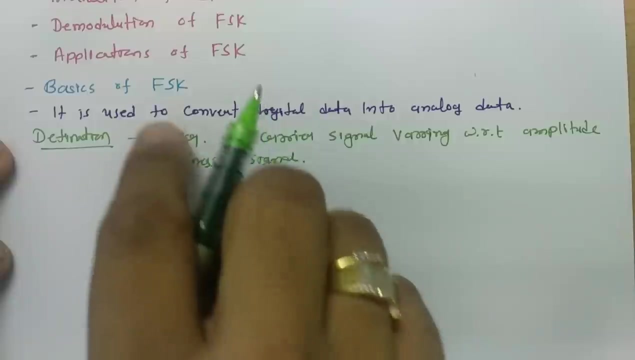 the amplitude of message signal, So frequency of carrier signal. we much Krishe pretty well, we know. So I told you. so it was frequency instead of diarrhea signal, cara signal反 e speciall ja frequency on carrier signal varying of this definition, see fsk- is frequency shift king and that is what frequency of carrier signal. 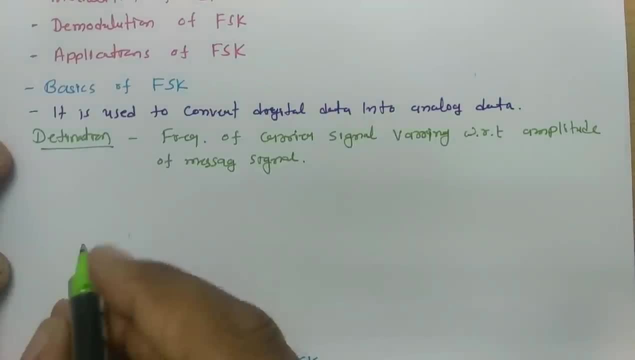 varying with respect to amplitude of message signal. so let us have first digital message. so we have a digital message. let us say it is empty, so we have a digital message. i'm just writing it first: one zero one, one zero z. so this is what the digital message that we have. 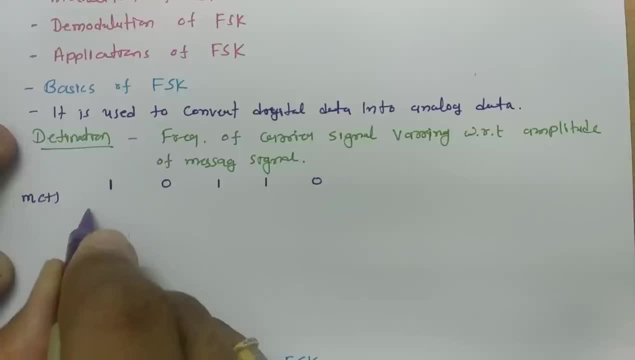 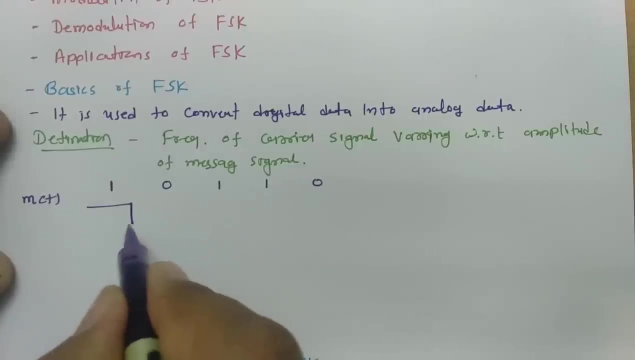 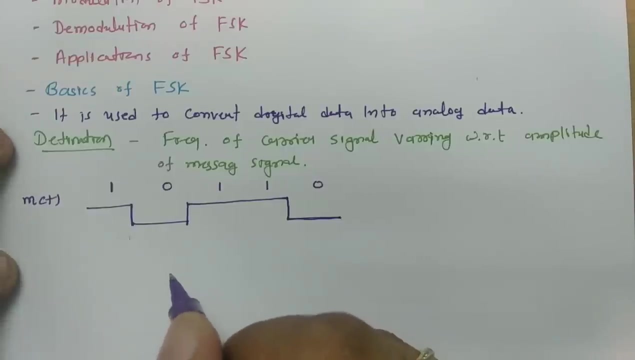 if you translate that in terms of waveform, then for one there will be, for nrz you will be finding: for one there will be high amplitude, for zero there will be low amplitude. for one there will be high amplitude and for zero there will be low amplitude. now see here in fsk frequency of 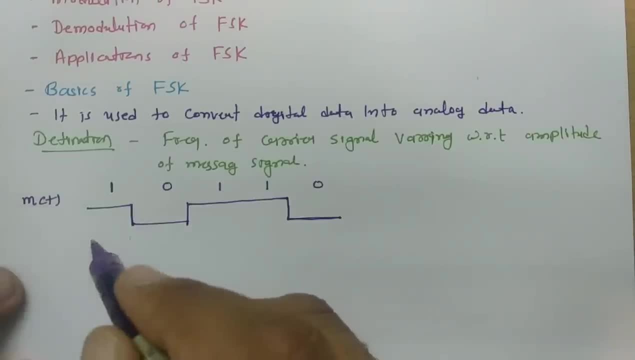 carrier signal that changes with respect to amplitude of message signal. so you'll be finding in fsk for binary. at first i'll give you example of binary fsk. so in binary fsk for one we send one frequency and for zeros we send other frequency. so if i say 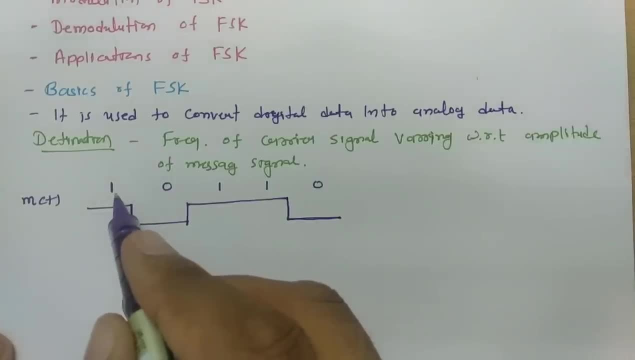 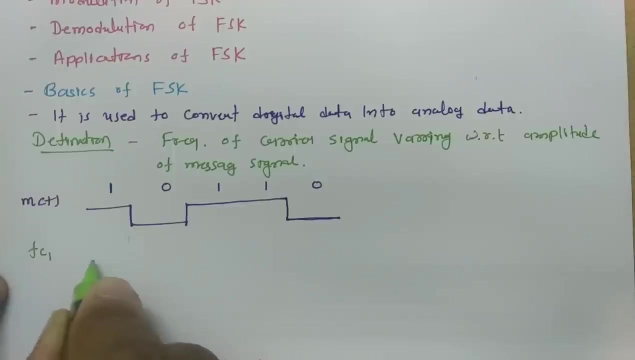 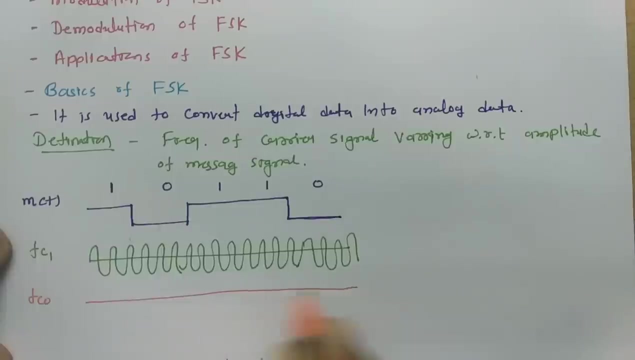 you for one if i said: if i send frequency fc1, carrier fc1, and for zero if i send frequency fc0. so let us draw waveform first. so here i have frequency fc1, and so here i have frequency fc1, and here i have frequency fc0. 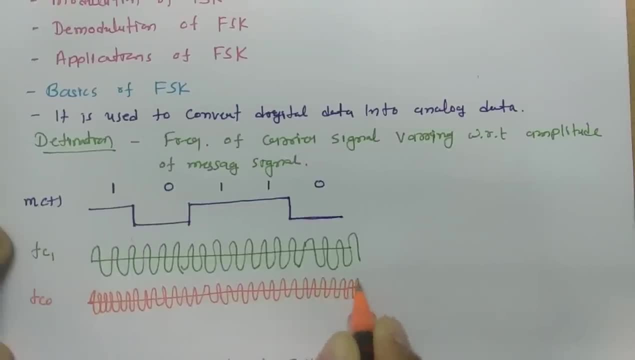 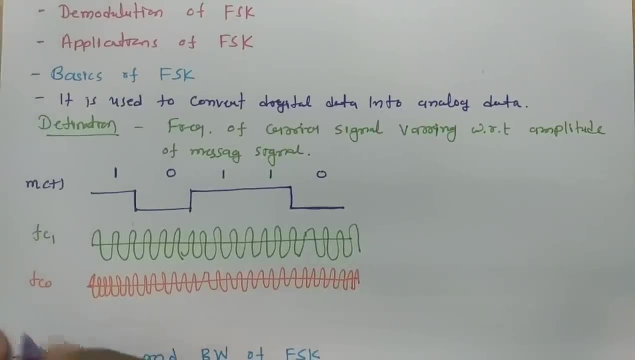 so when you have modulated signal, let us say it is two, which is phi of fsk, so in inch. oh, this sign onction is perfect when there is surnSurethy frequency of carrier signal that changes with respect to amplitude of message signal. now see, this is message signal when it is having one nz those. so for this instrument there is wrong faint sound that you have. 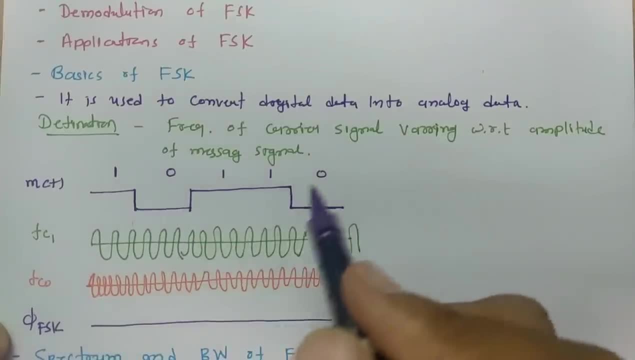 s. that is only one signal. clina bark, technical, that we found that theiyoruz measure of this frequency at input signal it's omission of sequence things of central d in amputation rate, except that here they are p, right now we're going fs and zero they. 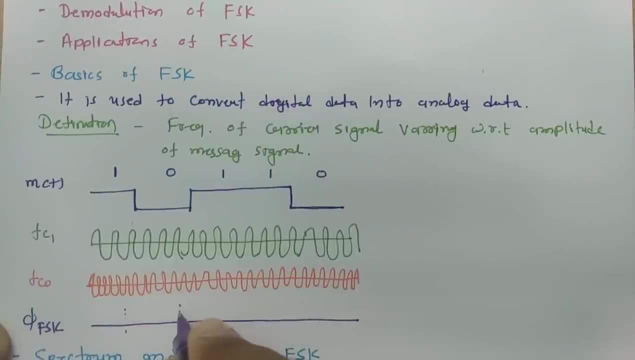 for this instant there is one right. for this instant there is one, and for this instant there is one, and for this instant, as well as for this instant, there is zero. so, as i have told in frequency shift keying, all we do is, for one, we send fc1- frequency and for zero, we send fc0. 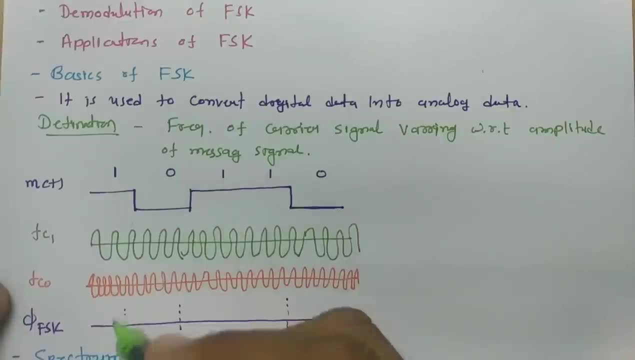 frequency. both frequency are different. so see, for this time interval, there is one, so we will be sending fc1 frequency. so that is this for this instant, even there is once. so here i will be sending fc1 frequency. and for zero, zeros, we will be sending fc0 frequency. so here there is zero, so we will be sending. 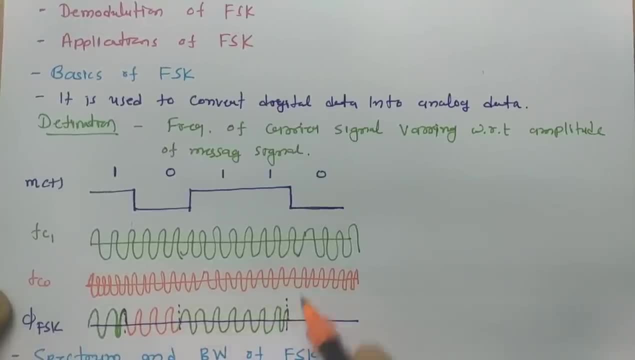 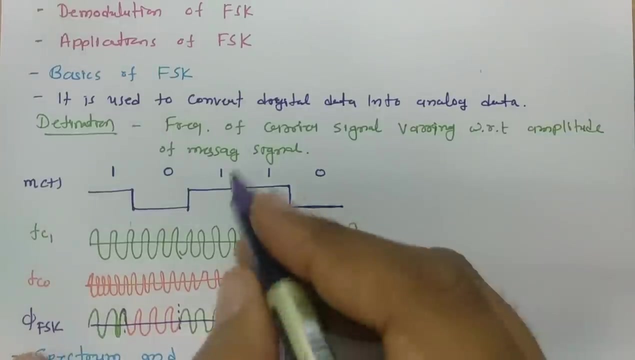 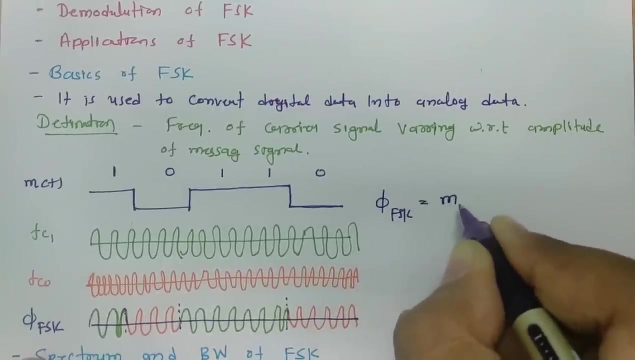 fc0 frequency and for this zero even, we will be sending fc0 frequency. so this is how we do frequency shift keying, where frequency of carrier signal, that is, changing with respect to amplitude of message signal. so as if you want to write a function of fsk, then that function will be. that function will be, let us say, for zeros, message signal is m0. 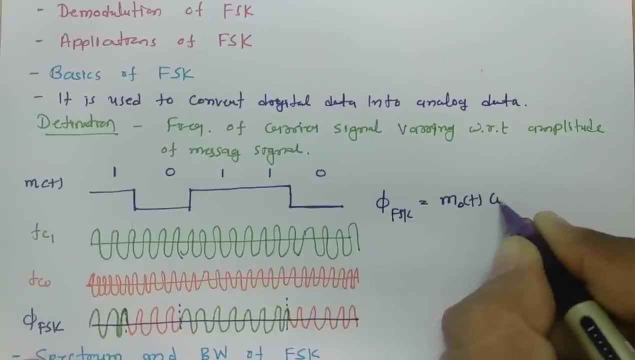 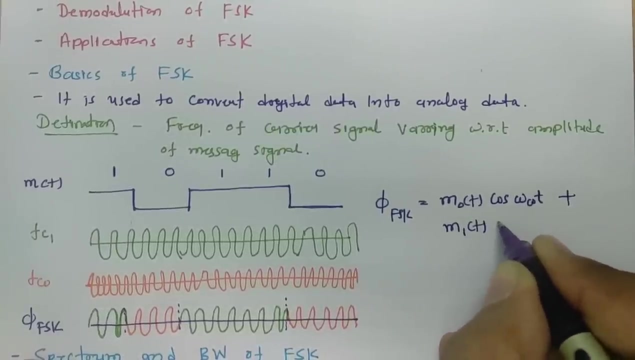 t. with that we will be multiplying cos of omega 0 ct, omega omega c0 t and for ones we will be sending, let us say, message m1 t into frequency cos of omega c1 t. so this is what the basic function that we perform in frequency shift keying, where 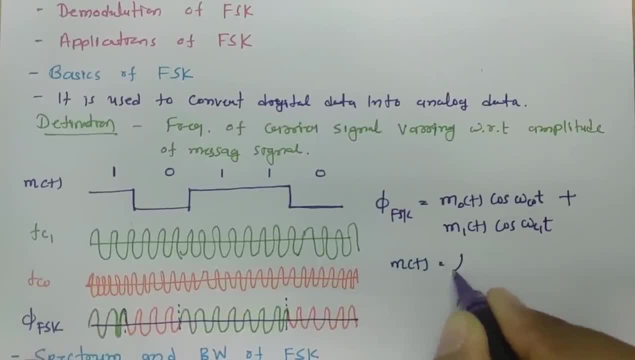 we can say message signal, that is, having one or zero. for one, we will be sending frequency fc1 and for zero, we will be sending frequency fc0. so this is what the basic thing that we perform in frequency shift keying. now let us try to understand a spectrum frequency. 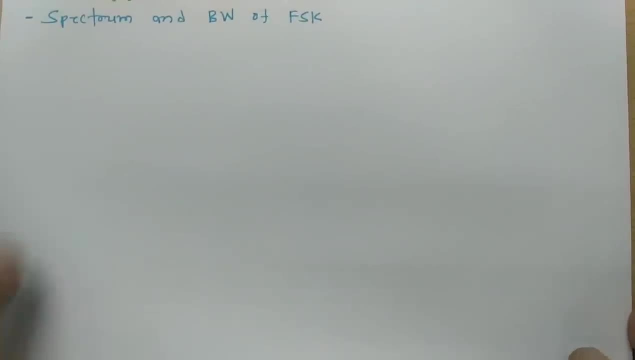 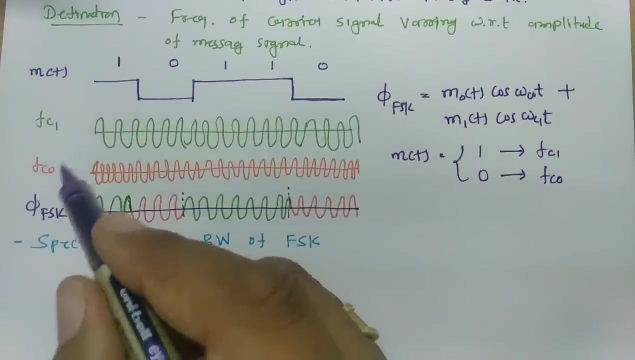 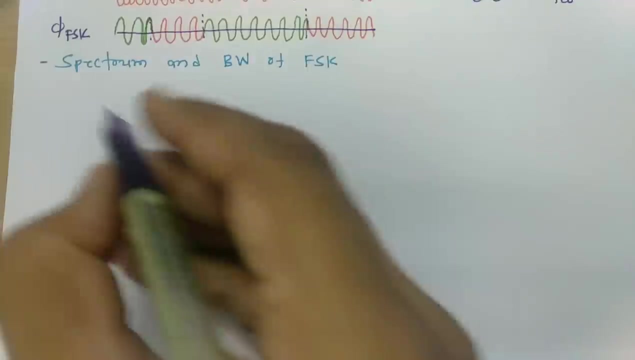 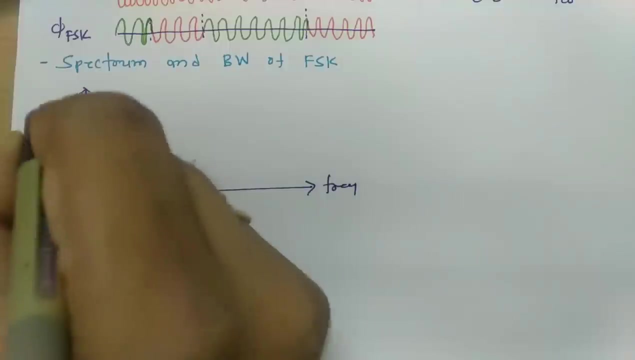 and bandwidth of fsk. so, as i have told, in frequency shift keying we send two frequencies: fc0 for zero and fc1 reveals 1s. so when you see its spectrum, when you see its spectrum, where here there is frequency, here there is amplitude and, let us say, frequency script king and would be sucked down��. 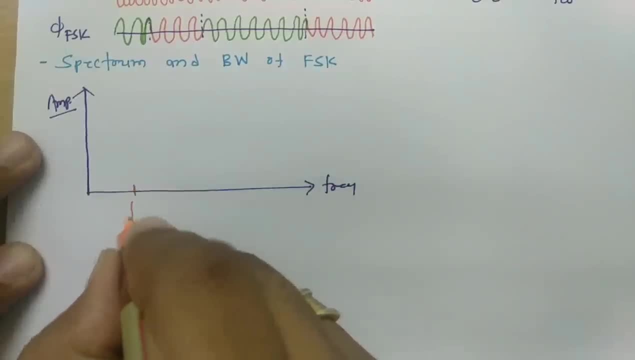 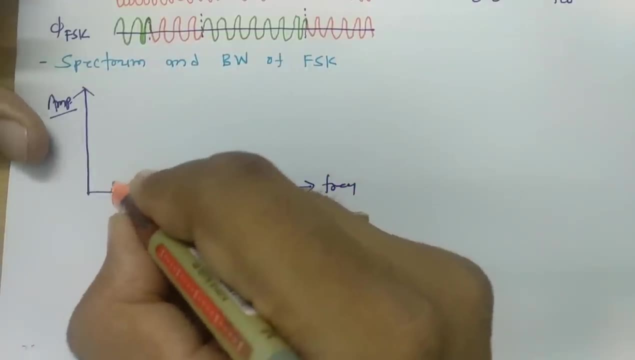 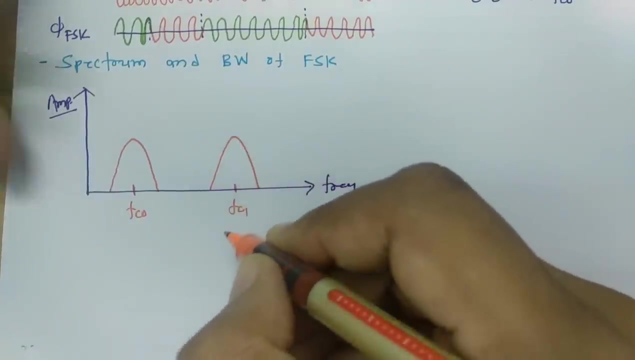 That means, when you see it in spectrum, where here there is frequency, here there is amplitude, and let us say, here there is FC0 and here there is FC1.. So this is what the band that we have for FC0 and this is what the band that we have for FC1.. Then for amplitude, shift king, we have seen. 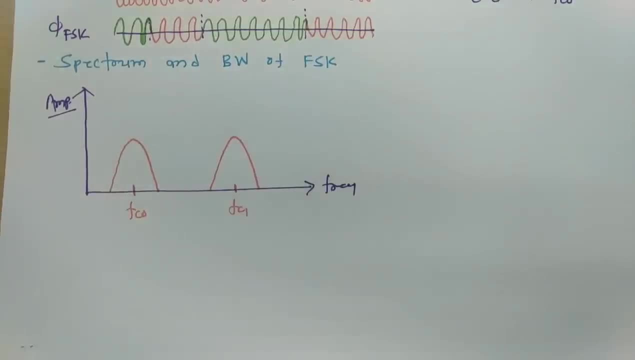 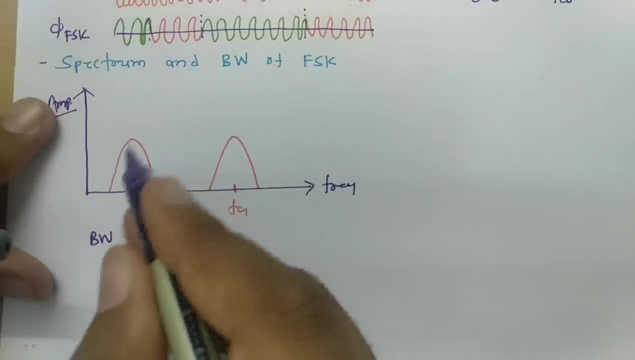 bandwidth for this individual band, Bandwidth for this individual band. I am not writing complete bandwidth Right now, I am just writing bandwidth for this band only So that we have seen. You can see my previous session of amplitude shift king, where you will be finding this bandwidth, that is. 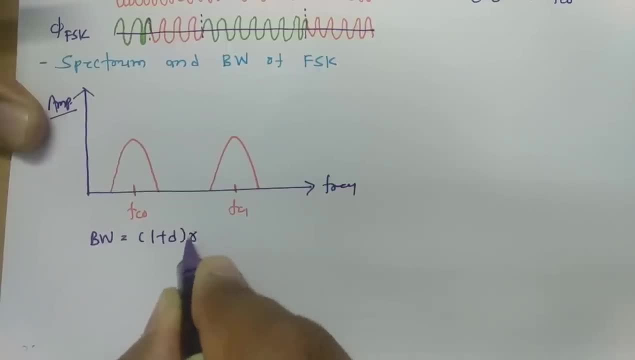 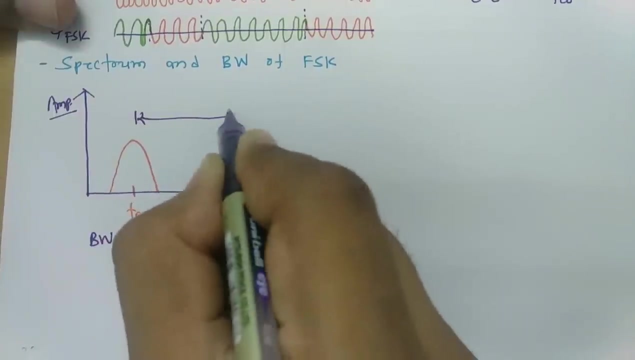 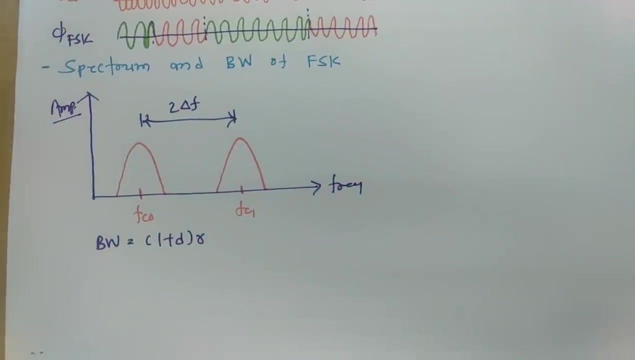 1 plus D into baud rate R. So this is what the bandwidth that is there with one band. Now see here the gap in between these two band, that is 2 delta f. Gap in between these two band, that is 2 delta f. So the total bandwidth. 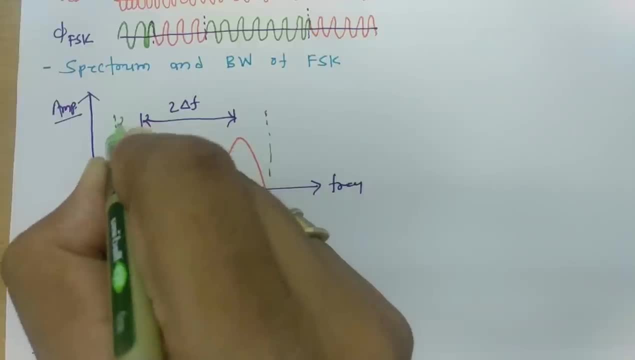 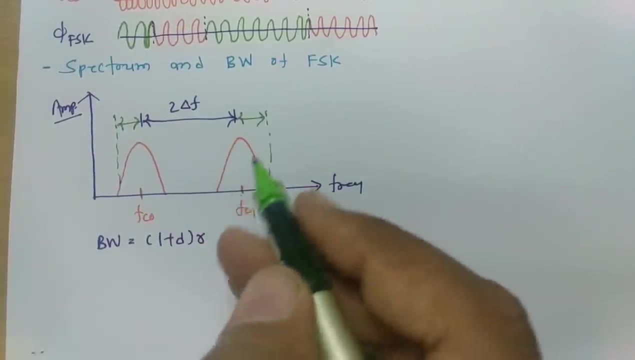 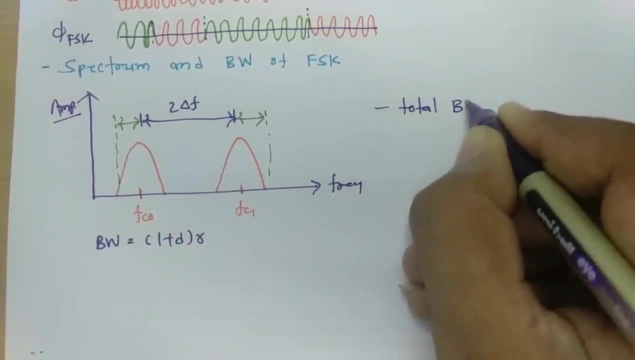 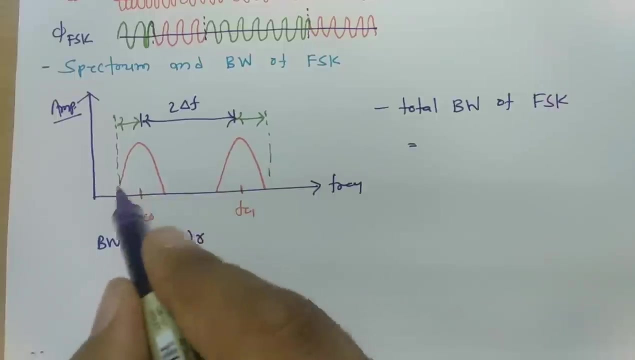 the total bandwidth of Fsk. that will be this bandwidth plus 2 delta f plus this bandwidth, So ultimately total bandwidth, total bandwidth of Fsk. So that will be See for this complete band. this bandwidth is 1 plus D into r, So this: 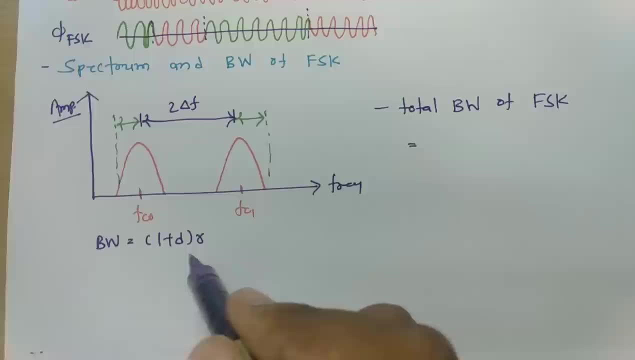 is what half band. So that will be half of 1 plus D into r plus 2 delta f plus half of 1 plus D into r for these half band Right. So total bandwidth will be 1 plus D into r by 2.. 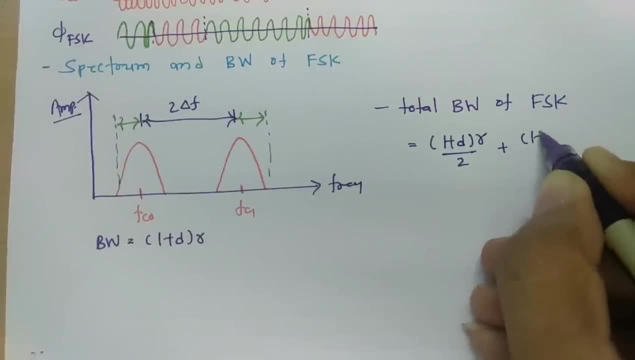 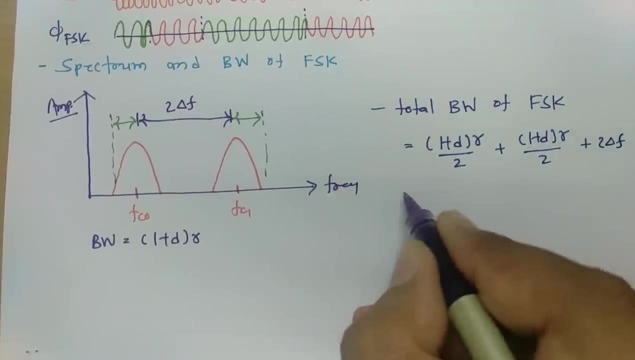 1 plus 1 plus d into r by 2 plus 2 delta f. So if you calculate this this half plus half, that will be 1 plus d into r plus 2 delta f. So see, this is what the total bandwidth. 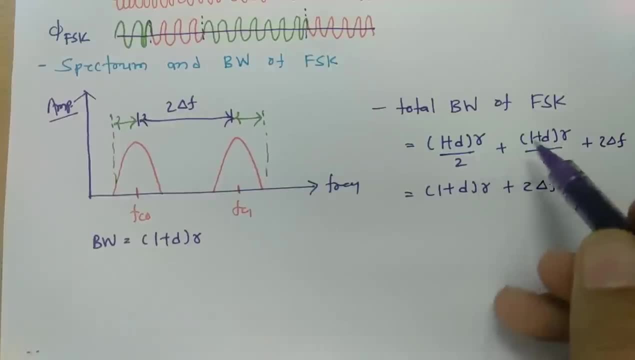 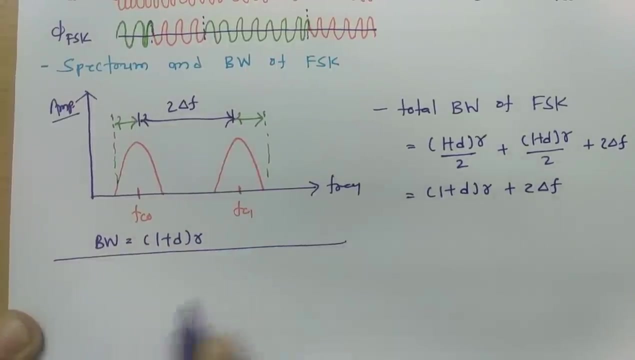 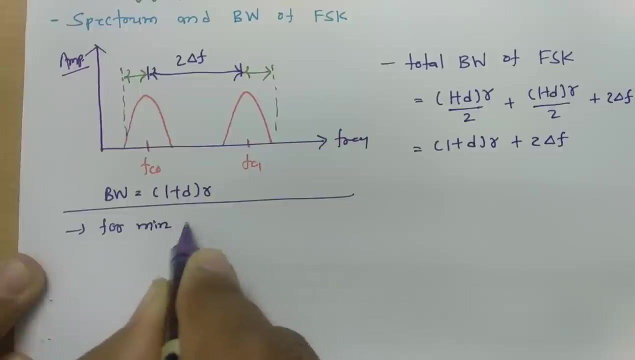 which is there with frequency shift king, And this is for binary FSK. Now see as, if I want to calculate minimum bandwidth, If I want to calculate minimum bandwidth, So for minimum bandwidth, for minimum bandwidth, see this: d, that is what modulation factor. 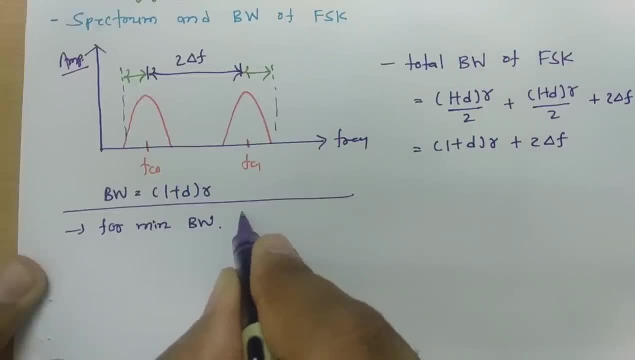 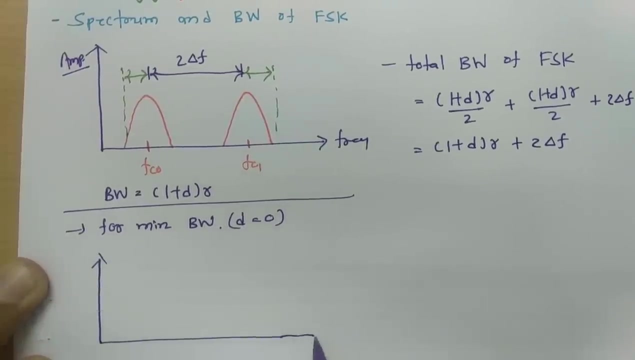 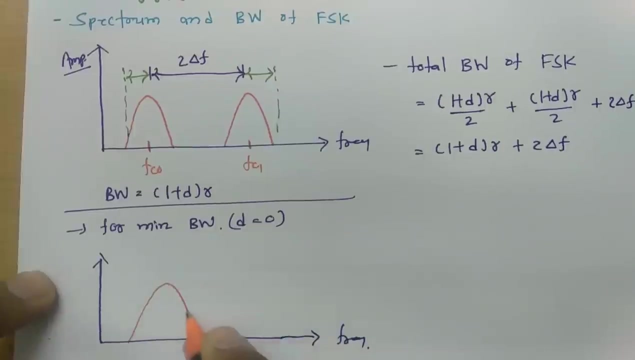 right. So for minimum bandwidth, you will be finding this d is equals to zero. So as if this d is equals to zero, and if you want to plot our frequency spectrum, then you will be finding that frequency spectrum that will looks like this: Both are just touched to. 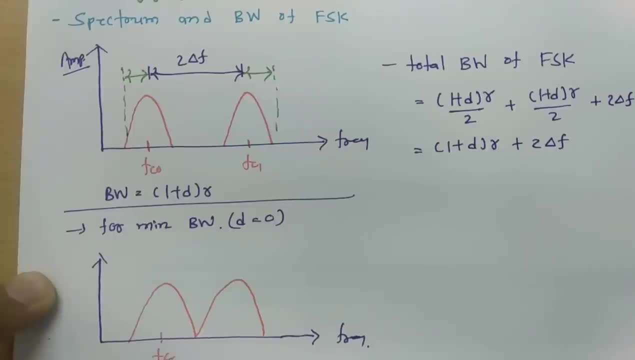 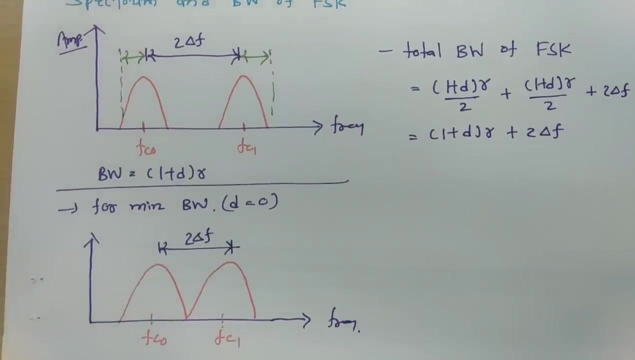 each other. Well, this will be f0, fc0 and this will be fc1.. And now we finding: this is what 2 delta f. This is what 2 delta f. So, for minimum bandwidth, d should be equals to zero, And it is what. 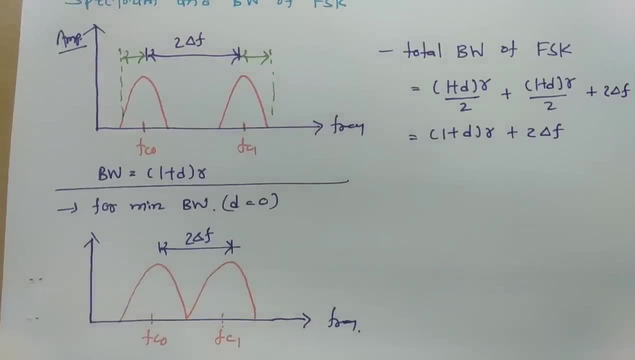 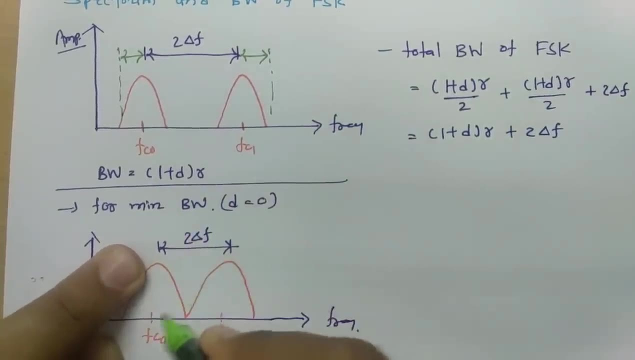 touching like this right Now. if you calculate this 2 delta f for minimum bandwidth- this was for minimum bandwidth- Then there will be actually half of this band plus half of this man, So that will be 1 plus d into r, And where d is equals to zero. So you'll be. 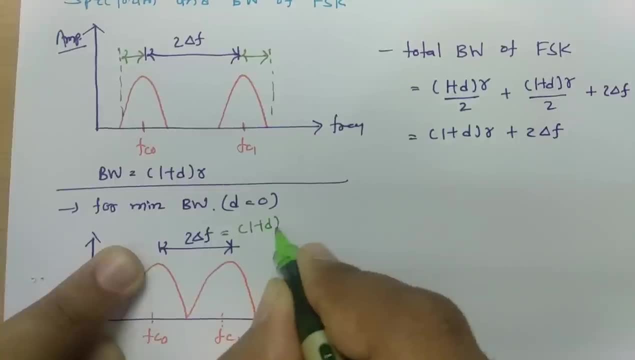 finding. this is what: 1 plus d into r by 2, plus 1 plus d into r by 2.. So that is actually 1. 15. 15. 16. 19., 20., 22. 22.. 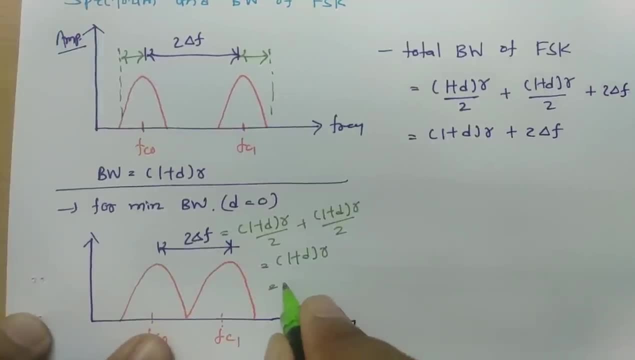 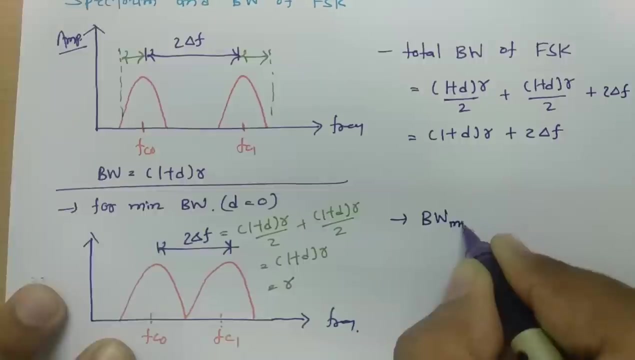 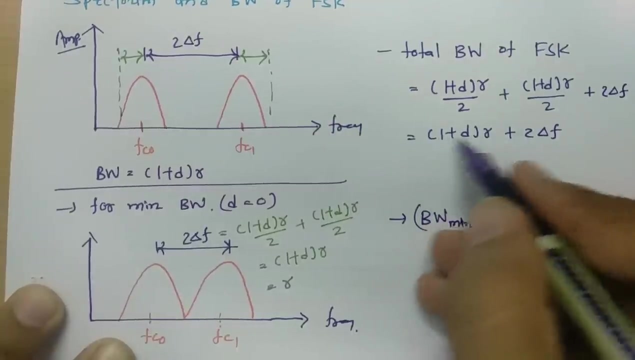 23. 24. 24. zero for minimum bandwidth, so it will be r. so 2 delta f, that is equals to r for minimum bandwidth. so for minimum bandwidth, 2 delta f, that is equals to r, where r is baud rate. so if you calculate minimum bandwidth, so bandwidth minimum for fsk, so that has to be this: d is. 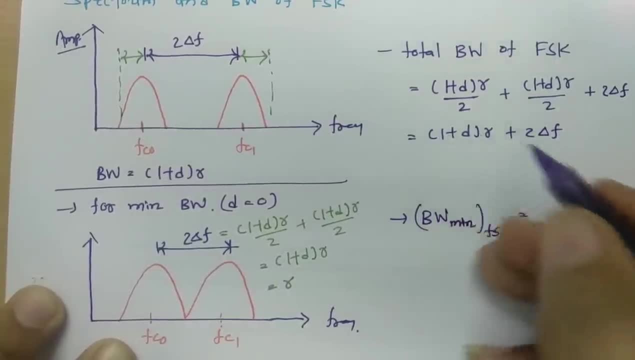 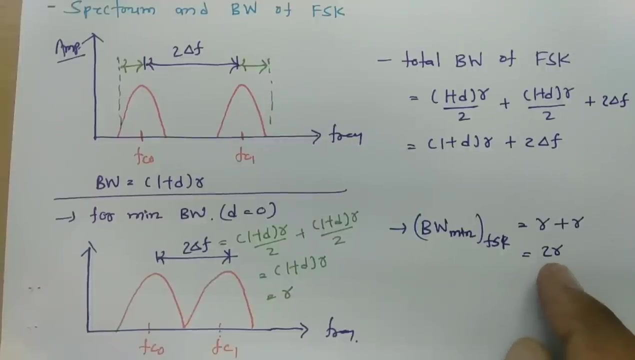 equals to 0, this d is equals to 0, so it will be r and this 2 delta f that is even r. so r plus r that is equals to 2 r. so minimum bandwidth: that is 0.. 2r for binary phase shift king. So ultimately now I think it should be clear how to have a. 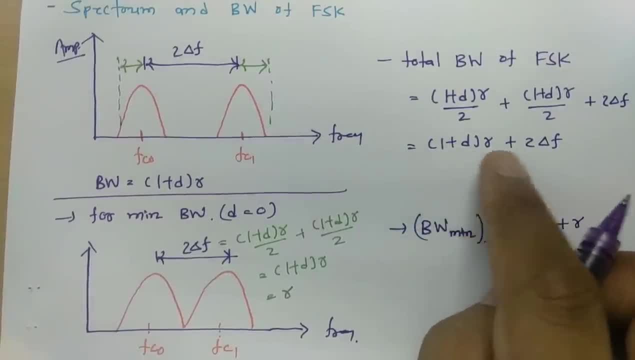 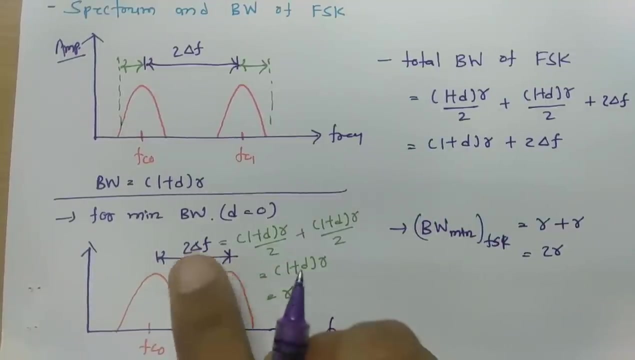 calculation of bandwidth. It is practically 1 plus d into r plus 2 delta f for binary phase shift king and minimum will be 2r, where r is baud rate and that 2 delta f, that is r. 2 delta f is what Spacing in between two bands. So spacing in between two bands, that will be r. 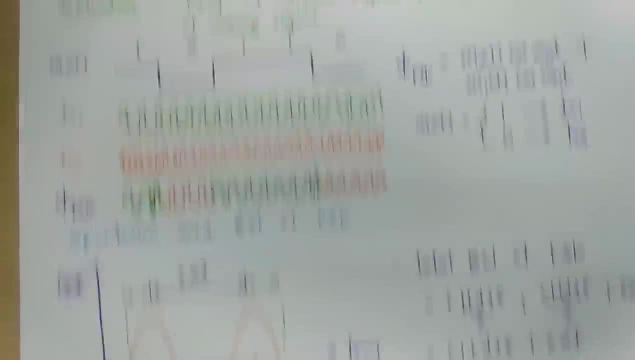 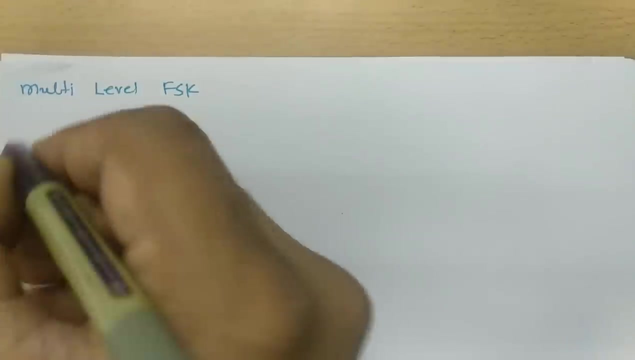 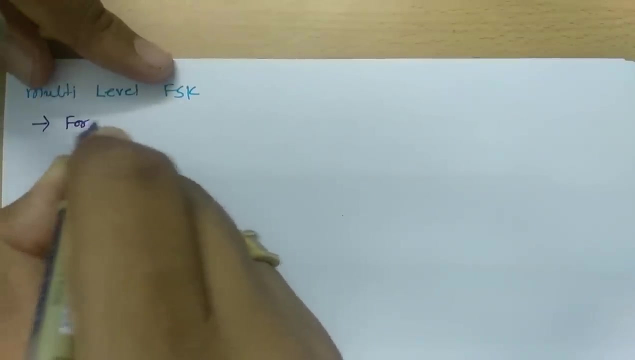 in case of minimum bandwidth. Now let us see multi-level FSK, So it will be more clear Now. see till now we have seen BPSK. So for BPSK, binary phase shift king, We have seen l is equals to 2.. If you compare this with 2 to the power n, then you will be getting 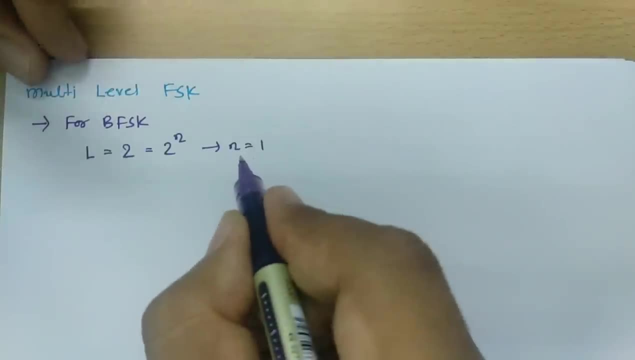 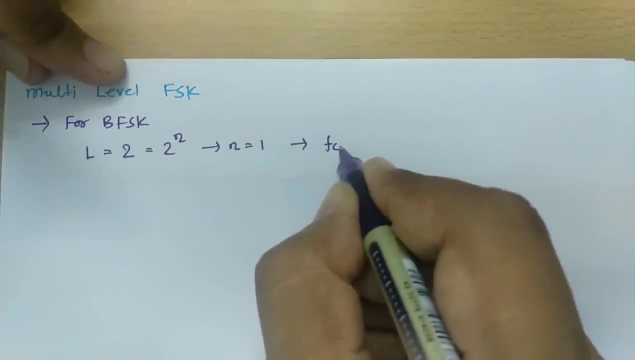 n is equals to 1.. So it means you will be representing levels by 1 bit. So if you represent n by 1 bit, total number of levels are 2 and for that you should be having frequency fc0 and fc1.. That is what we have seen till now. 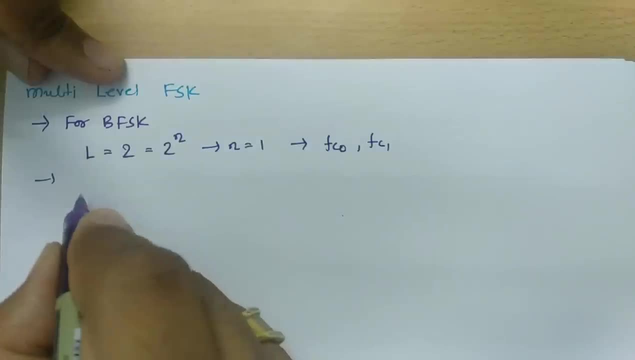 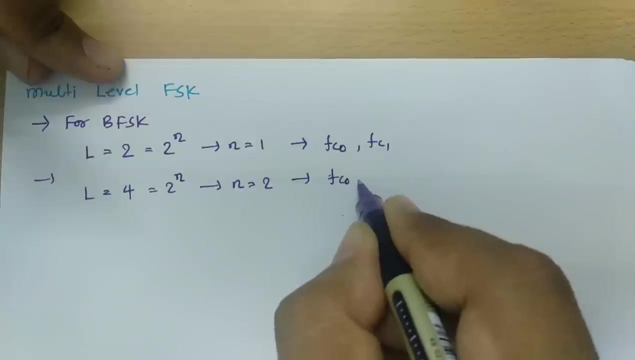 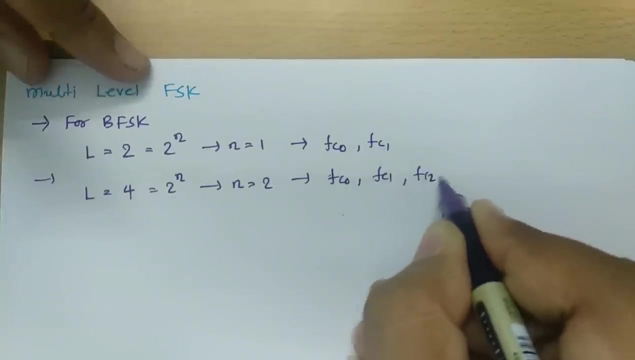 But for some other cases, like see if I say if l is equals to 4, what it means it will be 2 to the power, n where n is equals to 2.. So there are 4 levels means there should be 4 frequencies, 4 frequency spectrums, So fc0, fc1, fc2, fc3, that is, a 4 different frequency spectrum will. 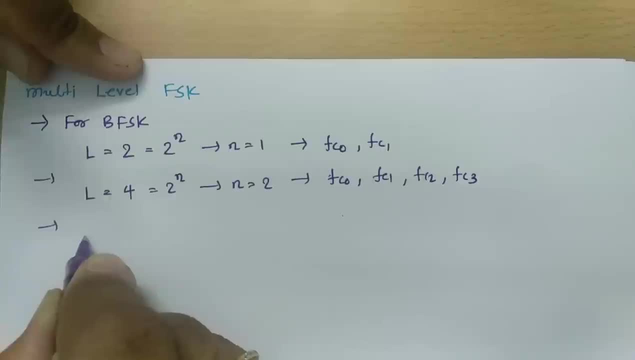 be there, for l is equals to 2.. So that is what we have seen till now. Another case that I am considering: if I say l is equals to 8. If you compare it with 2 to the power n, then you will be finding n is equals to 3.. Means single level represented by 3 bit. 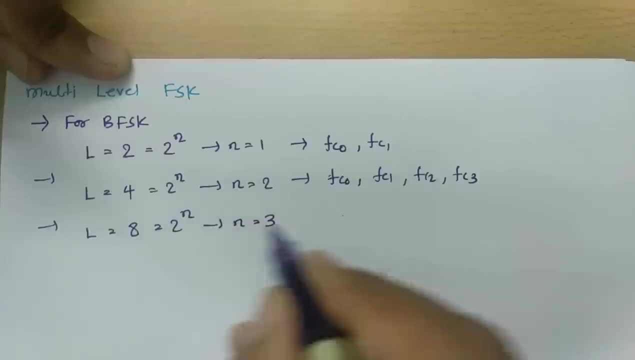 Total number of levels are 8.. It means there are 8 frequency spectrums. So there are 8 frequency carriers, So that will be from fc0, fc1 up to fc2.. So total 8 frequency spectrums are there. 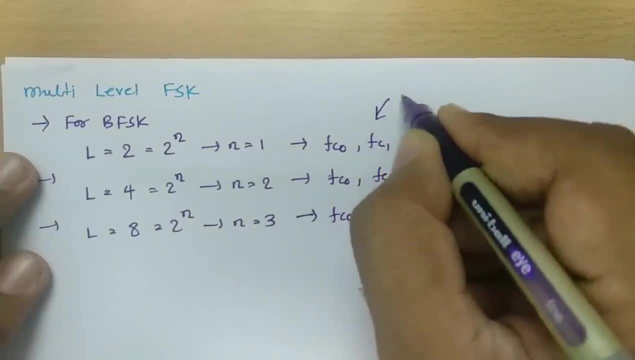 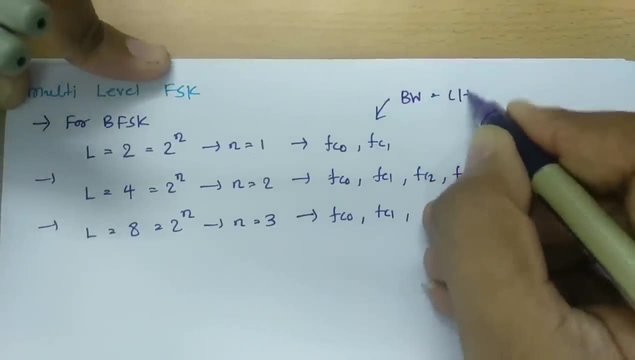 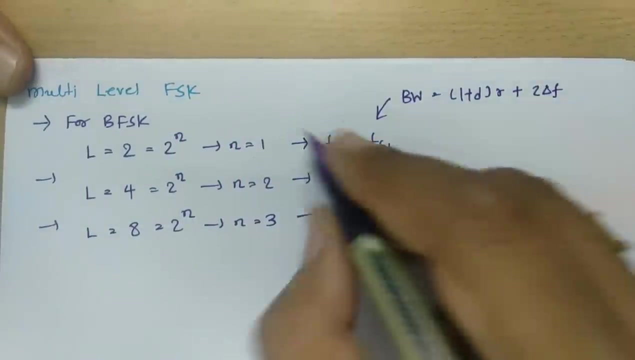 Now see for bpsk. for bpsk, we have recently calculated bandwidth, That is, we have recently calculated bandwidth that is 1 plus d into r plus 2 delta f. That is for bpsk, binary phase shift king, So for l level. now this is bpsk, So this is. 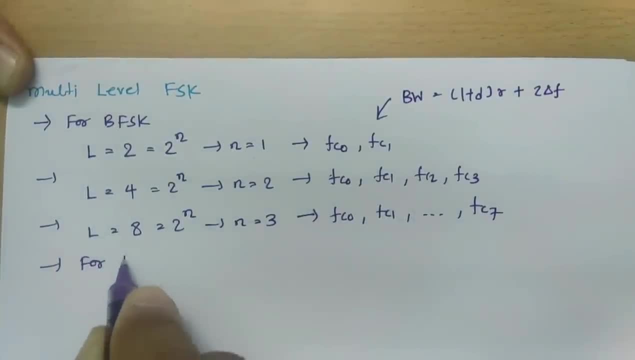 a binary phase shift, king. Now we will consider the ornithological space. So the binary phase shift here is this: So this will be that value here. Let's look at it: L level fsk- What will be bandwidth? So that bandwidth that has to be 1 plus d into r plus. 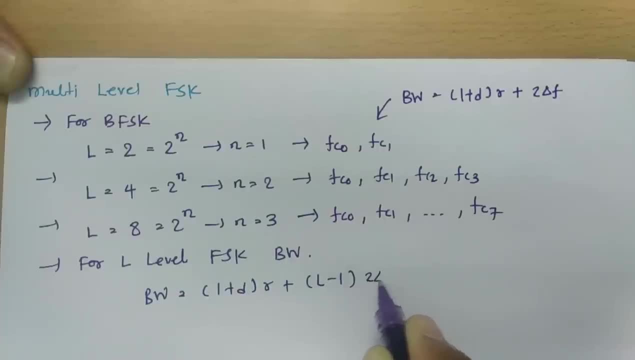 L minus 1 into 2 delta f. So that is what bandwidth for L level fsk You can see. compare it, for L is equals to 2, L, 2 minus 1, that is 1.. So that will be 1 plus d into r plus. 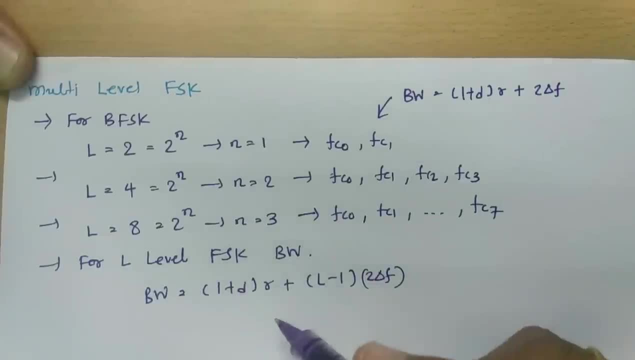 2 delta f. So that is how for L level it will be 1 plus d into r plus L, minus 1 into 2 delta f. that will be bandwidth for L level, fsk. And in this if you want to calculate minimum bandwidth. 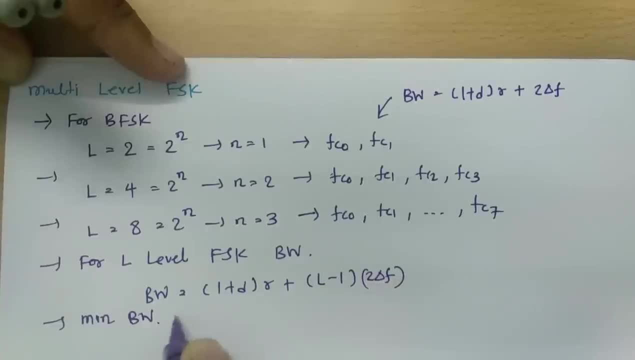 Minimum bandwidth. So for that d is equals to 0. And in that case your bandwidth will be 1 plus 0 into r plus L minus 1 into 2 delta f For minimum bandwidth. 2 delta f. that is r, So r plus L, r minus r, So that will be L r. 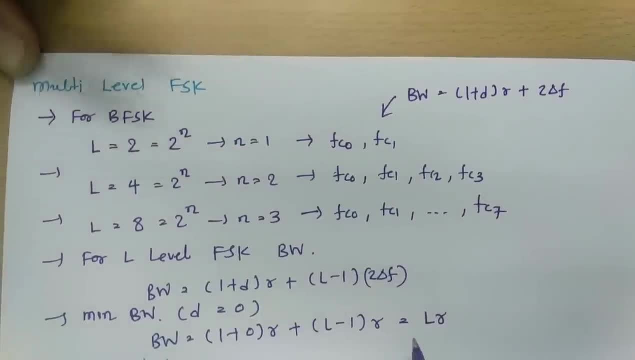 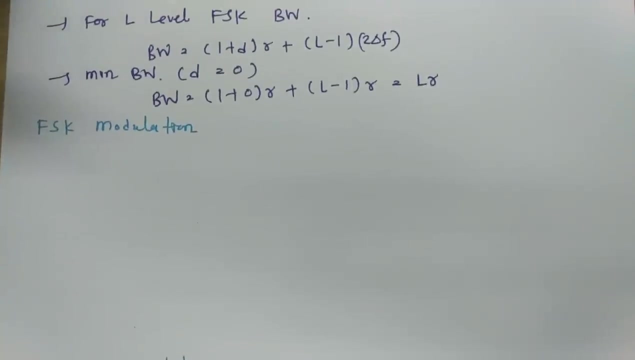 So minimum bandwidth, Minimum bandwidth for multilevel fsk, that will be L r. So that is how we can calculate multilevel bandwidth. Now let us try to understand how we can generate fsk signal. So fsk modulation Now see as: 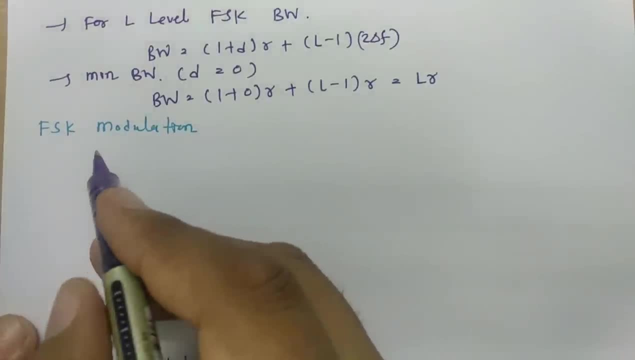 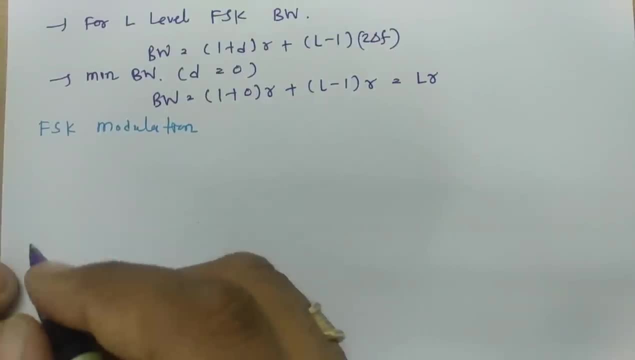 So fsk is equal to 0.. So fsk is equal to 0.. So fs blink gives you k tasks, So fk is equal to 0 in the� voluntary system, which I believe t equal to 0 in the multilevel class. 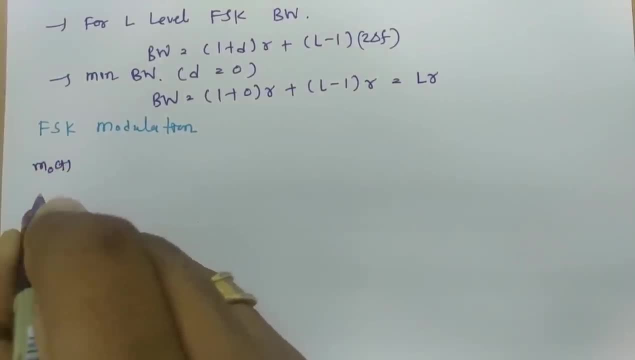 So fk is equal to 0.. So for multilevel we need to get, or at least click on the dash bar and find, our kLO in the multilevel class. So pk is 1 in the multilevel class, Very good. 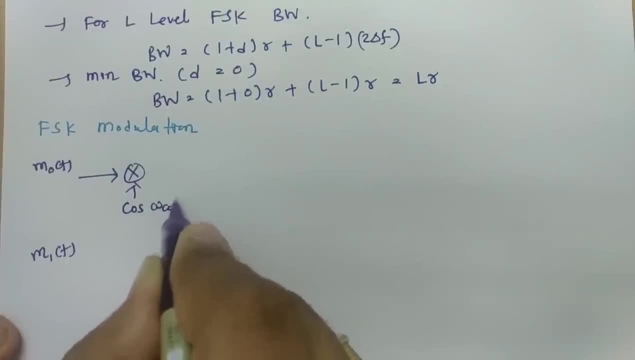 So 1 dot probe is equal to 0.. Now t is 10 to the power n into t, So 1 to the power n. So that is our kLO in the multilevel class Vbеть bit with frequency, cos, omega, c0, t, and for bit 1 you will have to multiply this with. 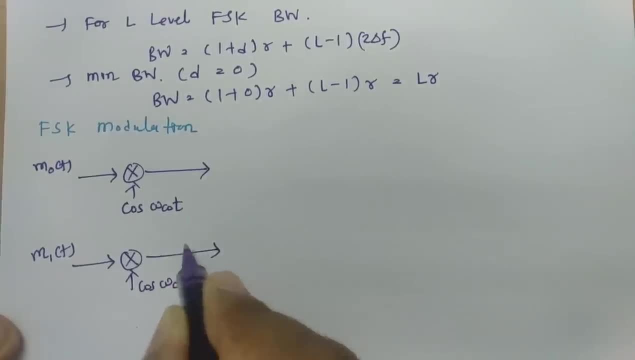 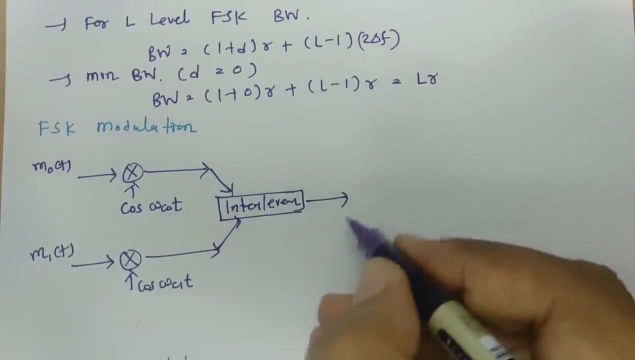 cos, omega c1 t. so you will be getting this and if you give it to interleaver, if you give this to interleaver, then it will be mixing this two signal and it will be generating fsk signal. and that fsk signal has to be m0 t into cos of omega c0 t plus m1 t into cos. 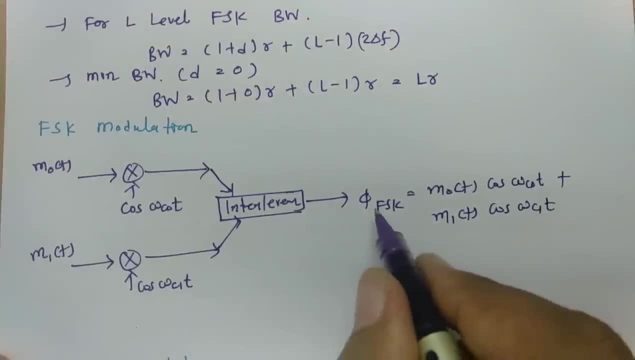 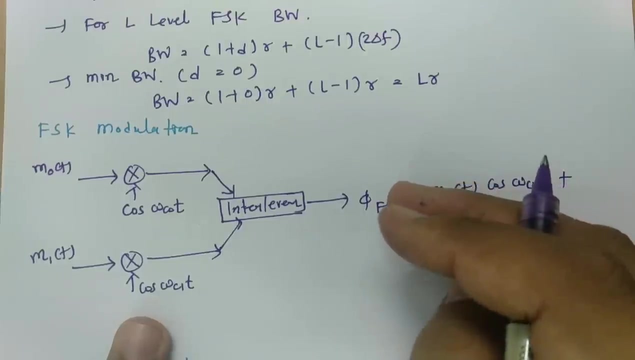 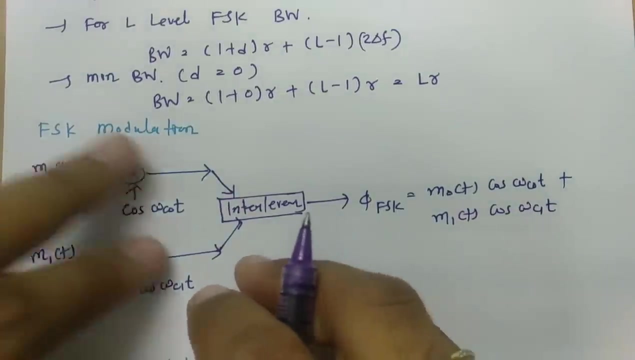 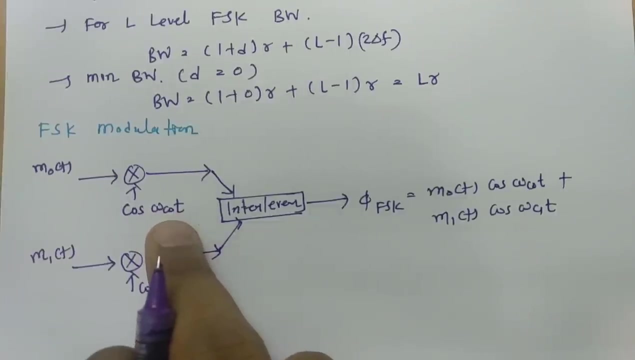 of omega c1 t. So you will be getting this. So you will be getting this. So you will be getting this f0 that we are sending and, for once, we are sending frequency fc1.. So that signal is fsk, which will look like this: 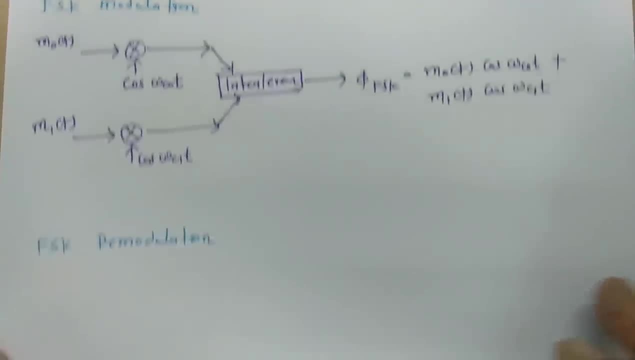 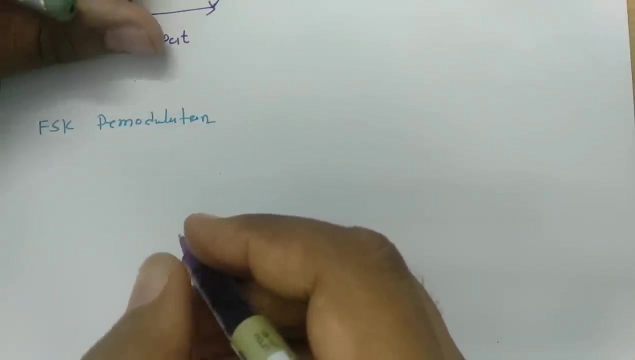 I think it is clear to all Now we should move on to fsk demodulation. So in demodulation there are two techniques. One is coherent and one is non-coherent. Now see for coherent. first I will explain. 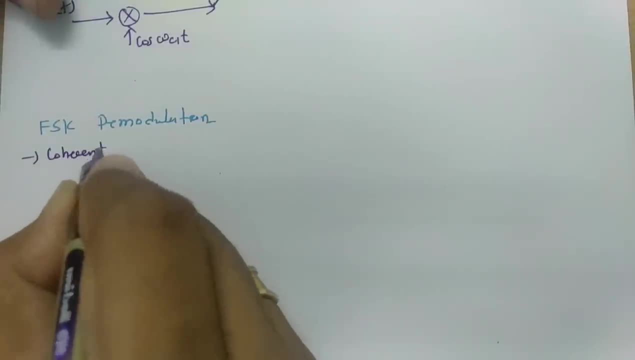 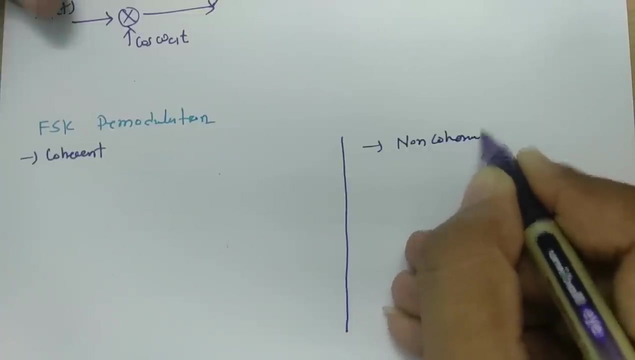 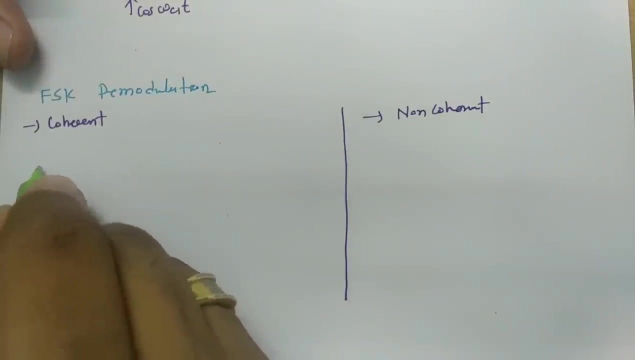 So coherent that I will explain first And then I will explain non-coherent demodulation technique. Now see in coherent modulation technique the signal which we receive, that we will be multiplying with two different frequencies separately. So here, if I say I have signal, 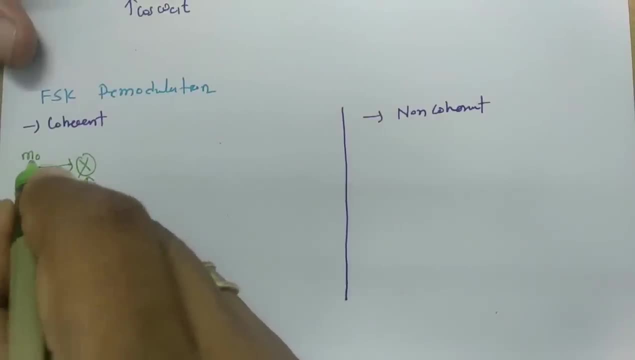 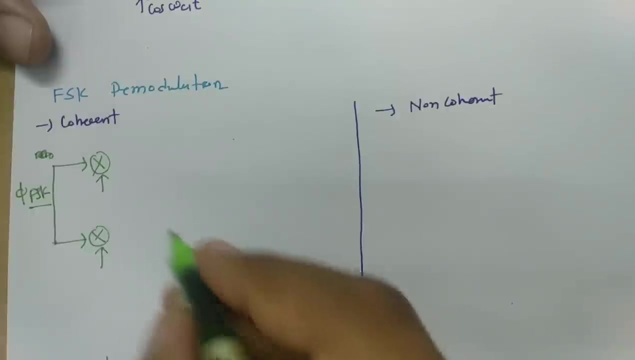 Right, And if I Have this signal, which is phi of fsk, So that is what I will be multiplying with cos omega c0 t and cos omega c1 t, So there will be two multiplication And if you pass this through low pass filter. 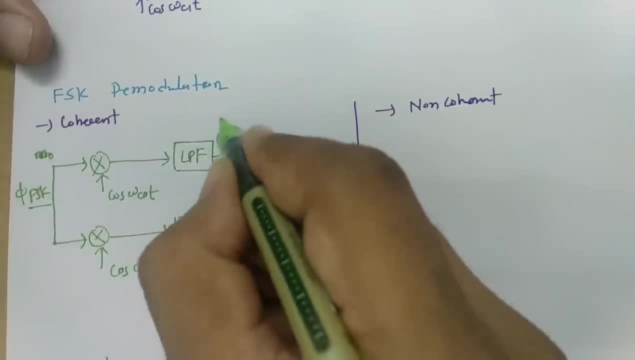 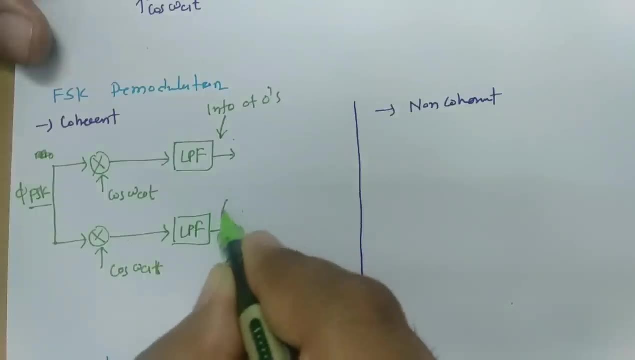 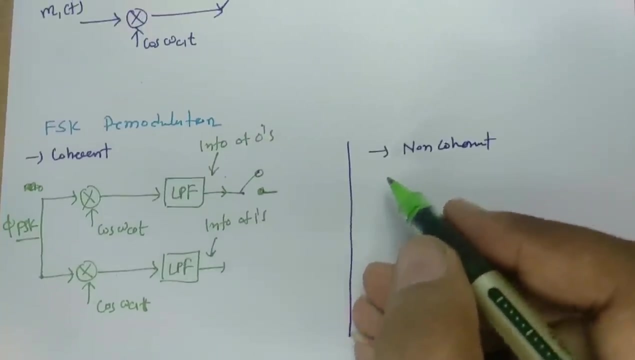 Then this will be having Information regarding zeros And this is having information of ones. Now all we will be doing is we will be giving it to sampler to deinterleave the signal. See, here we have interleaver Right, So it is having interleaving of two signals. 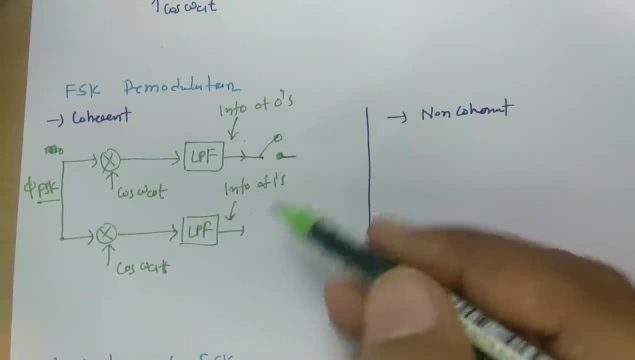 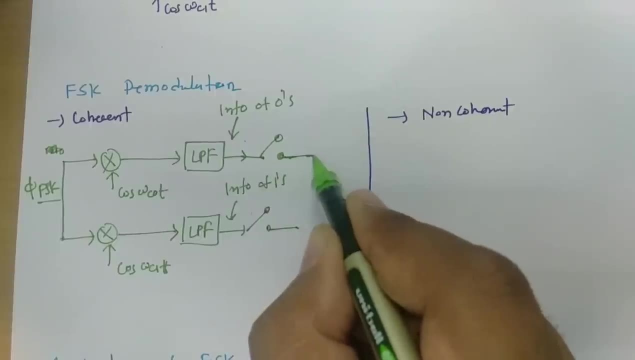 So now we need to do deinterleaving. for that We need to do sampling. So here I will be doing sampling And then I will give it to comparator block, And as if I give it to comparator block If this line is greater than this line. 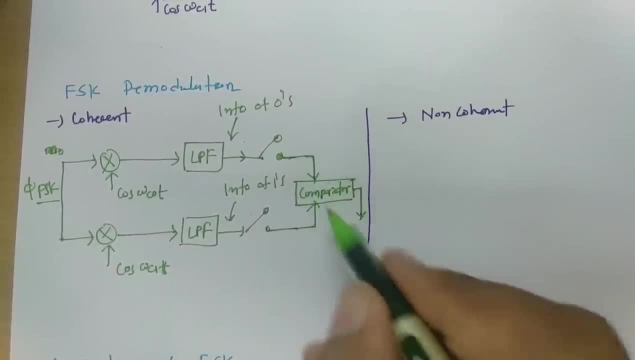 One can say: here zeros are there, And if this line is greater than this line, Then we can say: here ones are there. So here you will be having digital data Means empty. That is what digital data. So by having coherent demodulation, 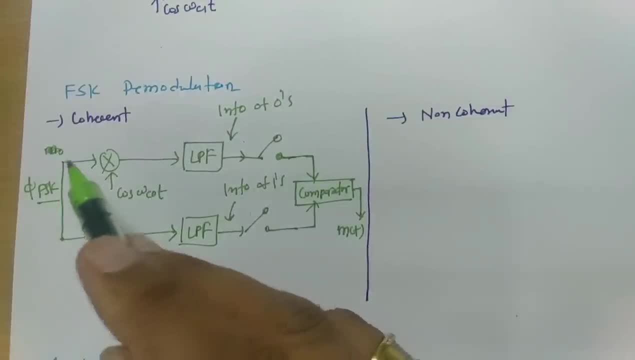 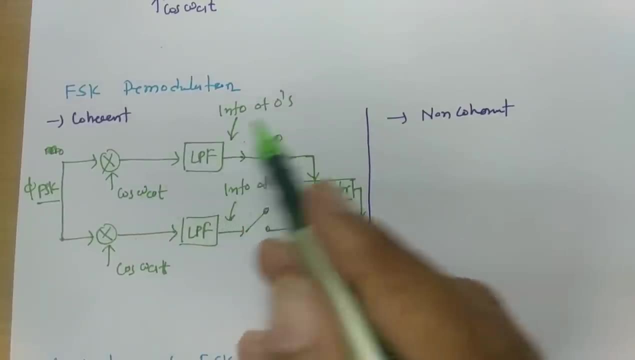 We need two carriers, Which we will be multiplying it with received signal And then pass it through low pass filter. Omega c0 will gives you information regarding zeros And omega c1 will gives you information regarding ones And by having Samples. 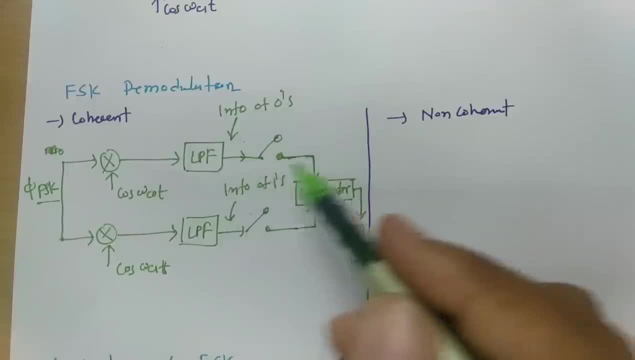 Compare both of the signals And if Zero signal is greater than one signal, Then you can say empty is having bit zero, And if once is having magnitude greater than zeros, Then one can say comparator is having output which is bit one. In non coherent we will be doing same thing, but oscillator or carriers. 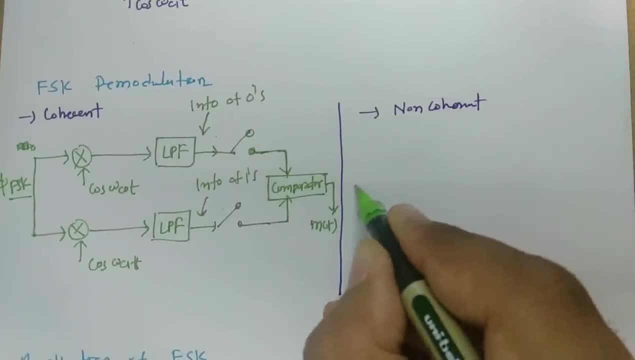 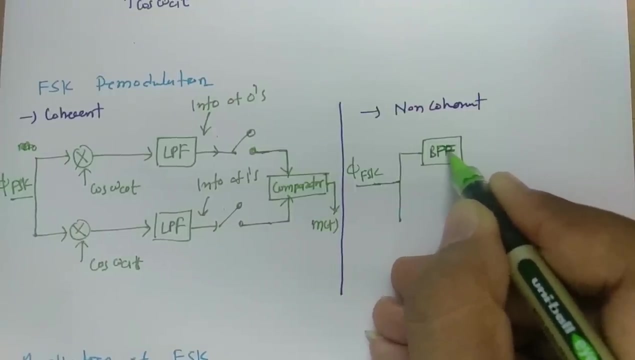 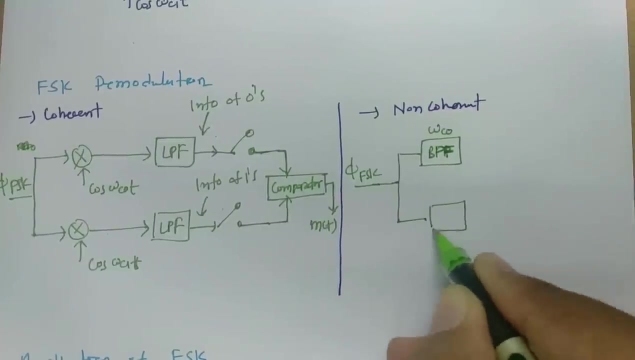 So, in non coherent, all we will be doing is we will be, having received The signal that is fsk, Then we will be giving it through bandpass filter And this bandpass filter that is having frequency fc0. And here we will be giving it to bandpass filter. 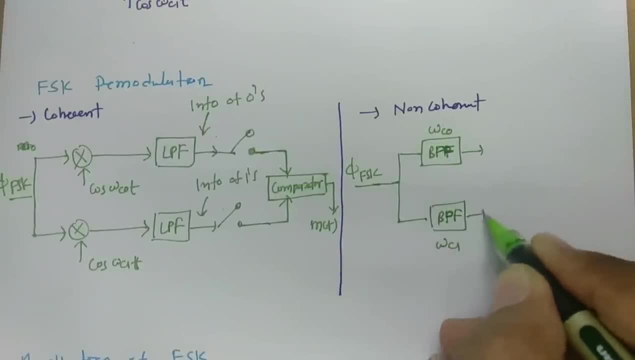 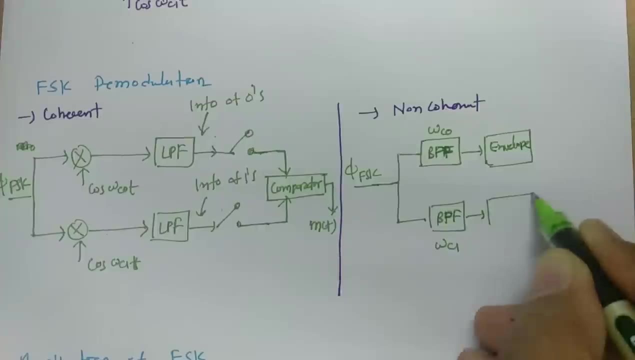 That is having frequency fc1.. Then we will pass it through envelope detector. So once you pass it through envelope detector, This will be giving you idea about zeros. Then sample it And then give it to comparator As you do it over here.